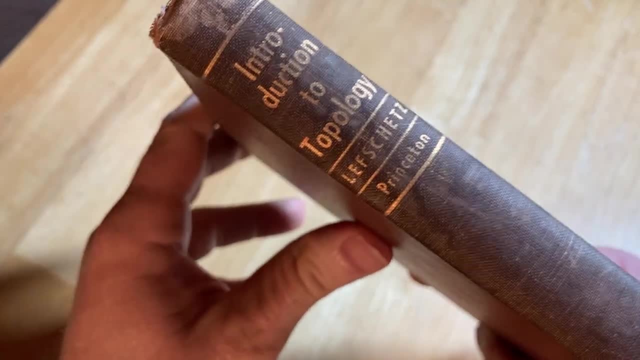 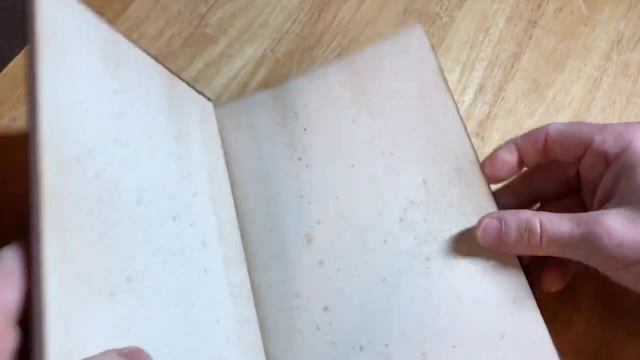 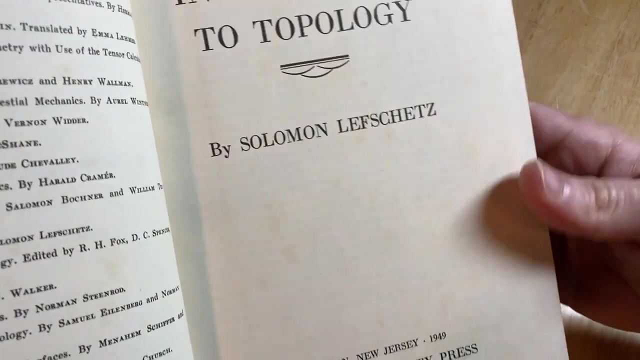 Here we have a book on topology, Introduction to Topology, Lefschetz, Princeton. it says: Let's open it up And it looks very, very old By Solomon Lefschetz, Princeton, New Jersey, 1949, Princeton University Press. 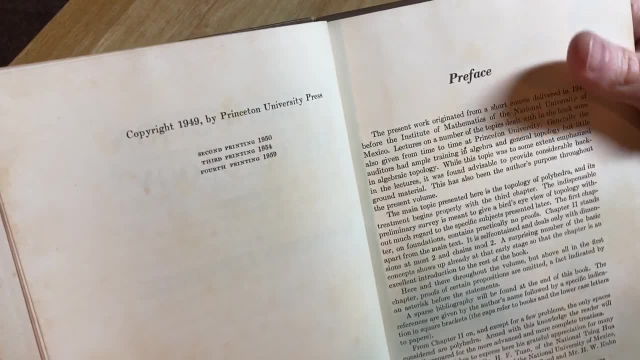 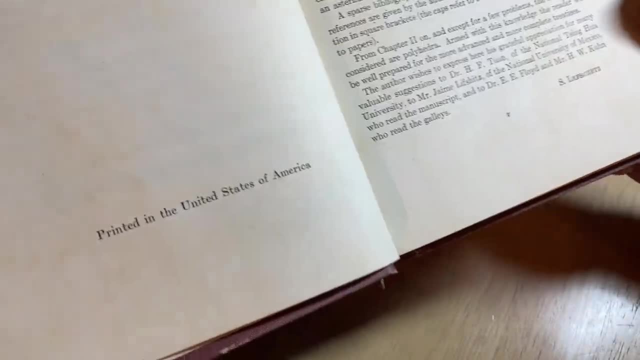 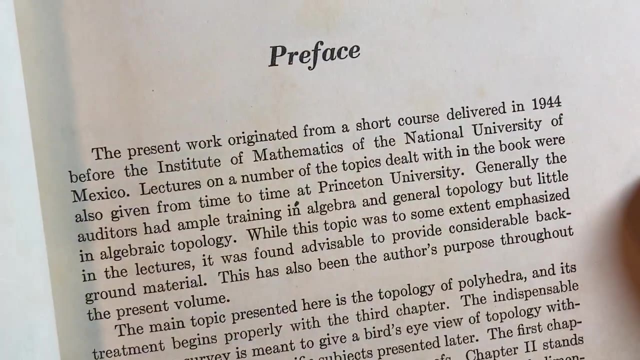 Really old: Copyright 1949.. And then this appears to be perhaps the fourth printing, because it says 1959.. Printed in the USA. Let's see what it says here. The present work originated from a short course delivered in 1944 before the Institute of Mathematics of the National University of Mexico. 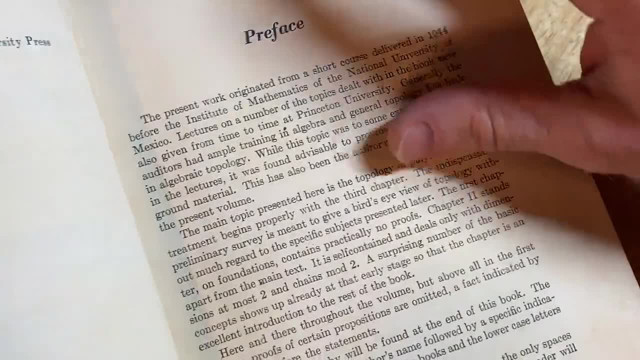 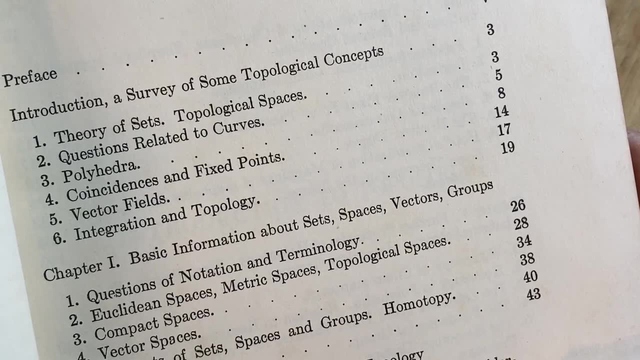 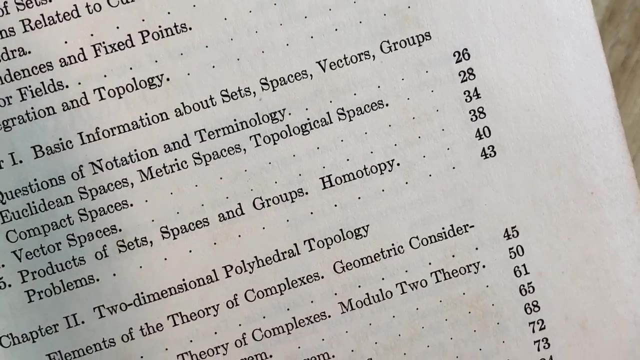 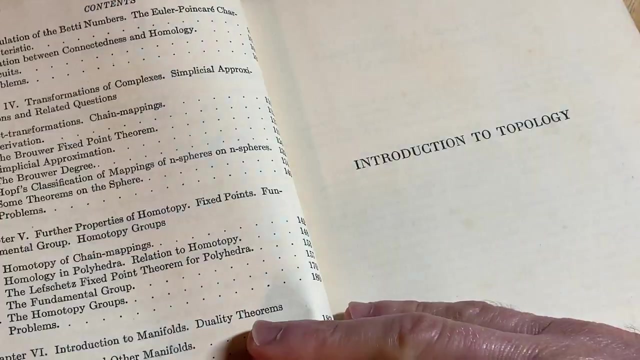 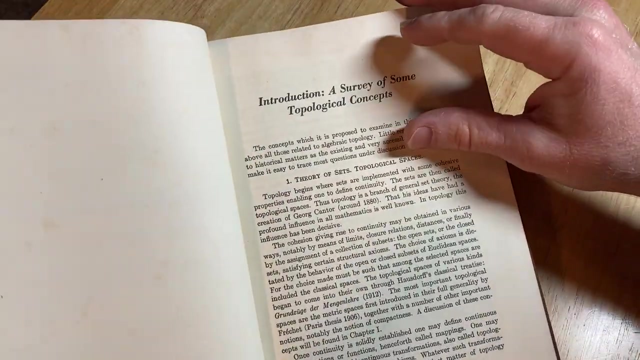 Okay, cool. So it starts with a survey of some topological concepts, Basic information about sets, spaces, vectors and groups, Some more topics here, And it's meant to be an introductory topology book. So, in theory, if you have the inclination and the background and the desire to learn topology, 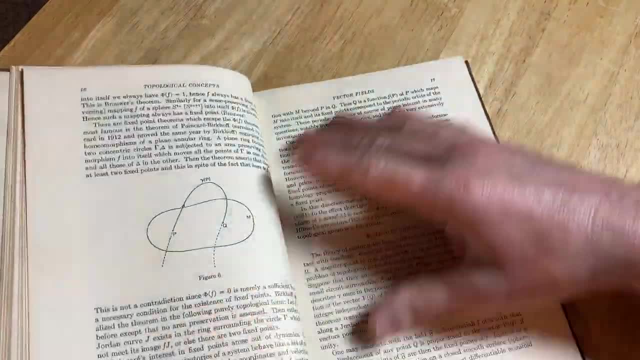 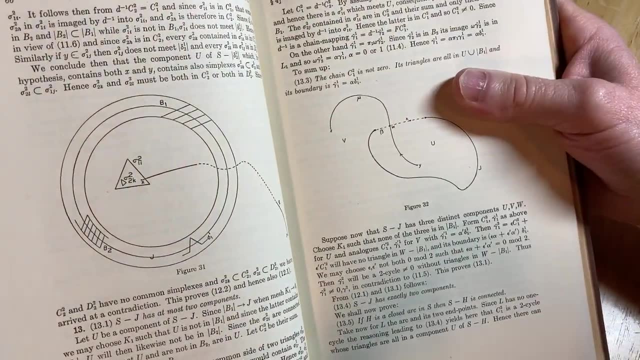 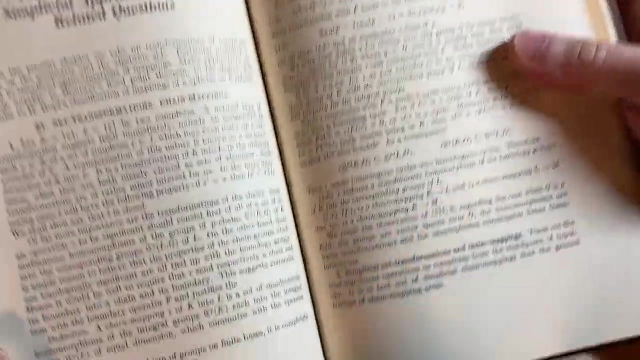 you could. You could, in theory, pick up this book and use this to learn topology. There are other topology books that are also good, perhaps better than this one, But yeah, this is an old book. I'm going to give it a whiff here. 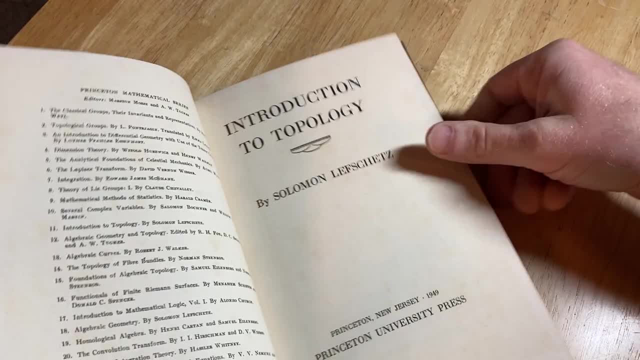 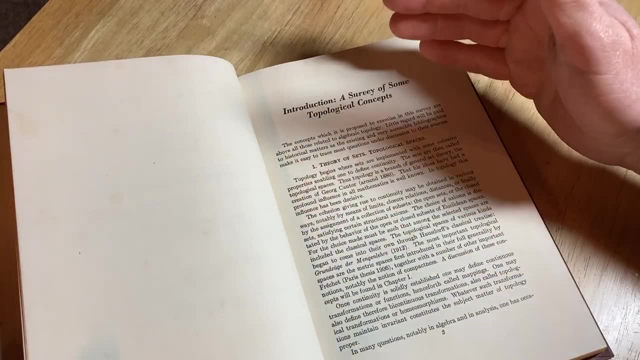 Just Old school book, right? If you can get a copy, I say definitely get a copy. I'll look for a copy, see if I can find one. If I can find one, I'll leave a link. I'll leave a link in the description. 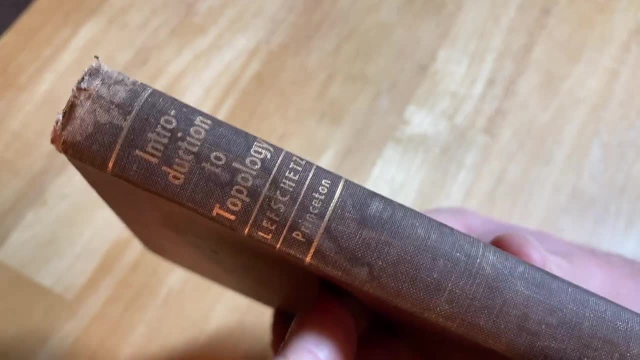 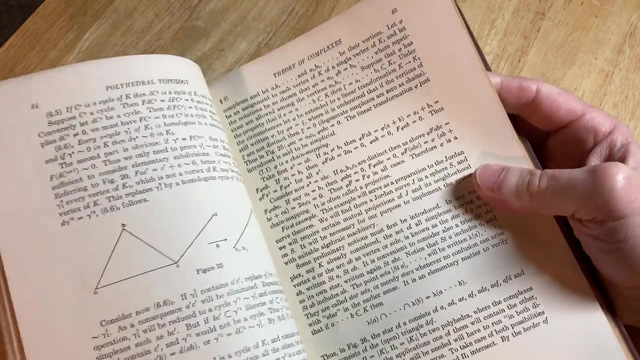 But I don't know if I can find a copy of this book. It's I don't know how common. it is Pretty cool, though, Old old school topology books. You have these old books and you can use them to learn new knowledge. I think that makes it really cool.